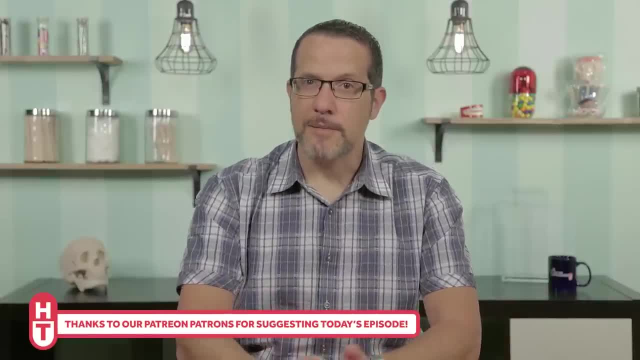 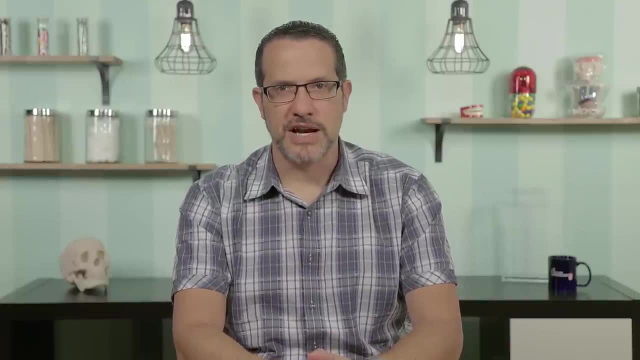 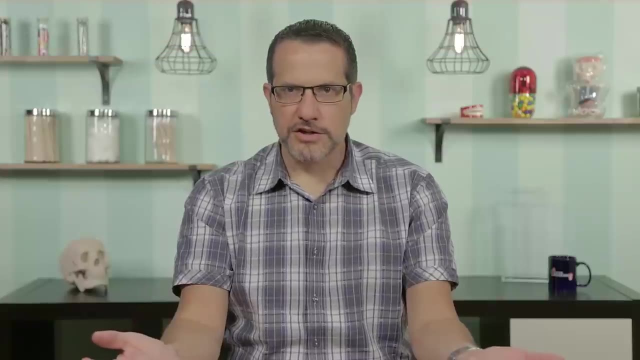 We asked, you answered. As a Patreon perk, many of our patrons voted for an episode on the dangers of sitting. This has been in the news a lot recently. It's also the topic of this week's Healthcare Triage. There's a wealth of literature that shows that sitting can be linked to obesity or being. 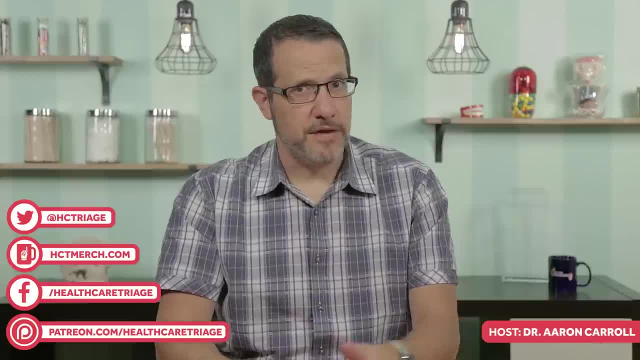 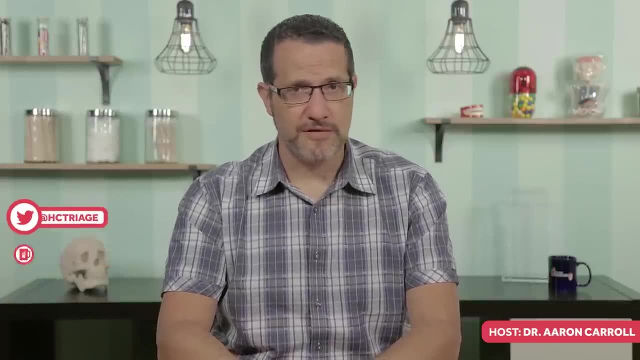 overweight, And of course, those things can be associated with bad health outcomes. But what's concerning is that, even after you control for those things, it appears that sitting is still really bad for you. For instance, a study published in 2009 in the journal Medicine: 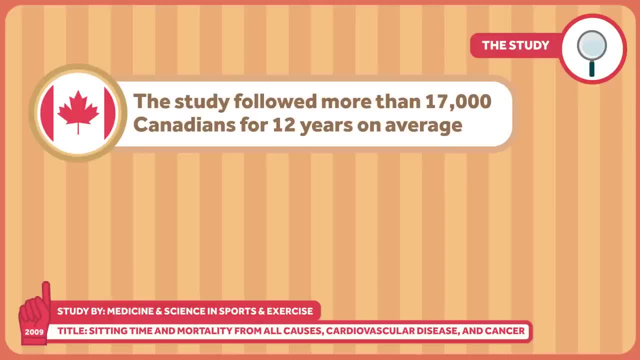 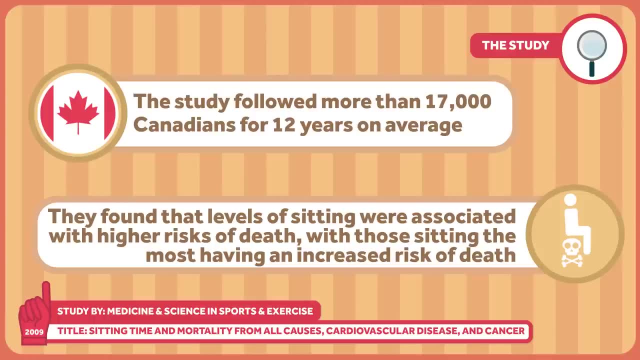 and Science in Sports and Exercise followed more than 17,000 Canadians for 12 years. on average, They found that levels of sitting were associated with higher risks of death, with those sitting the most having an increased risk of death of more than 50%. In fact, the 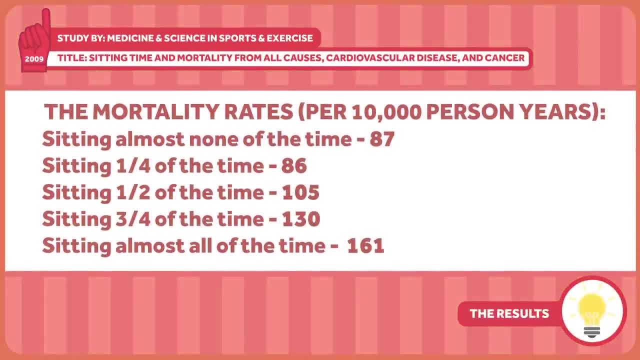 mortality rates for those who sat almost none of the time, one-fourth of the time, half the time, three-fourth of the time and more than 50% of the time were associated with more than 50% of the time where 87,, 86,, 105,, 130, and 161 per 10,000 person-years. Those 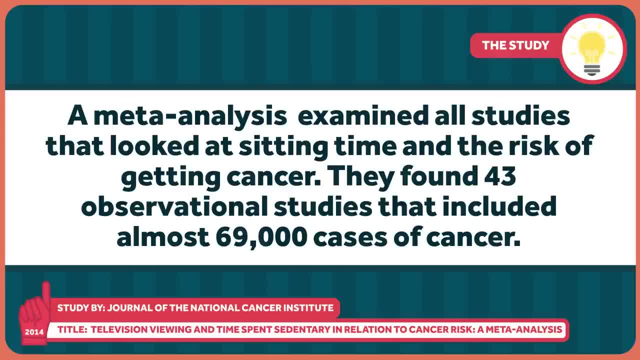 differences are scary. A meta-analysis was published just two years ago in the Journal of the National Cancer Institute that examined all studies that looked at sitting time and the risk of getting cancer. They found 43 observational studies that included almost 69,000 cases of cancer. 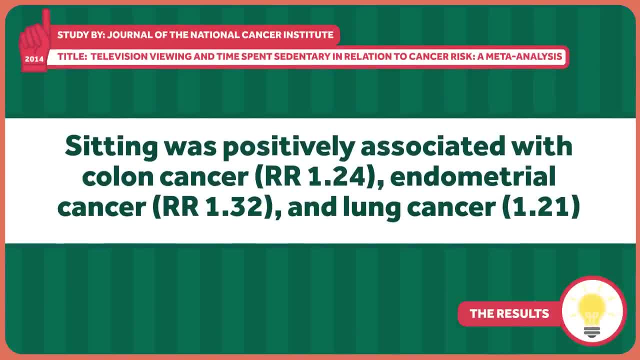 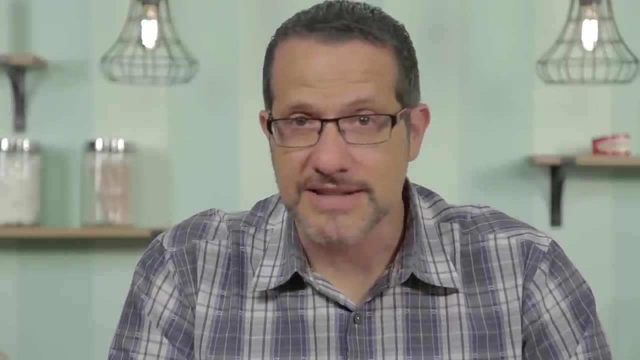 And the news wasn't good. Sitting was positively associated with colon cancer, colon cancer and lung cancer and lav jewel cancer. Here's where it gets really badAdjusting for physical activity made no difference. This means that even those who tried to exercise couldn't wipe away the dangerous associations. 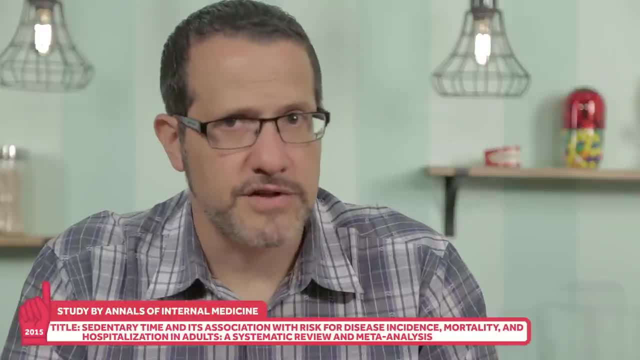 of being sedentary. A meta-analysis published this year in Annals of Internal Medicine reviewed 47 articles that looked at sedentary behavior while adjusting for physical activity and found It was very others that got sick, but only 48 in it. They then had 75trl authors أى the target because 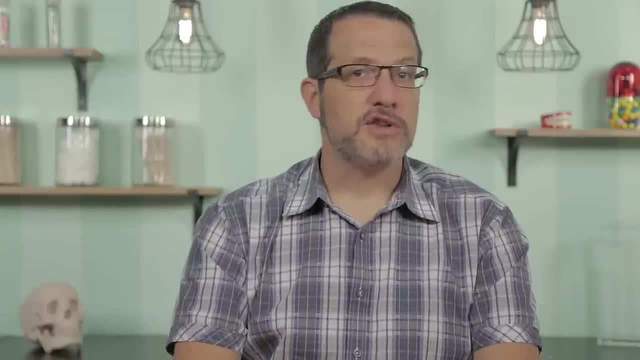 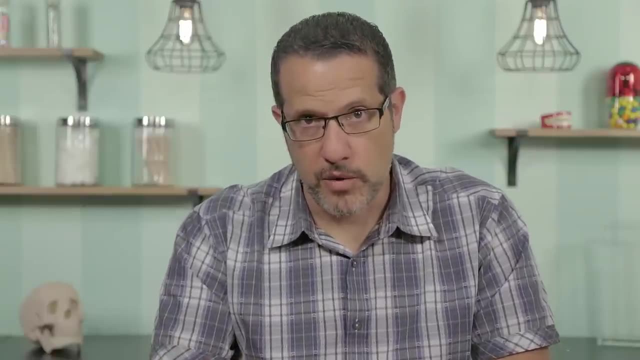 lace workers had problems with cutting Entre, read dienteins' blood count or perderered the found that more sitting was associated with increased all-cause mortality hazard risk of 1.24,. cardiovascular disease mortality hazard risk: 1.18,. cardiovascular disease incidence hazard ratio: 1.14,. 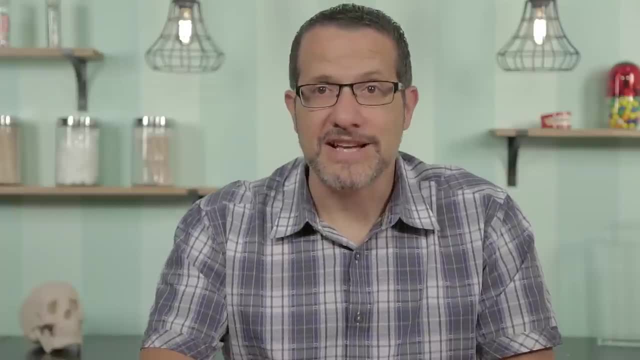 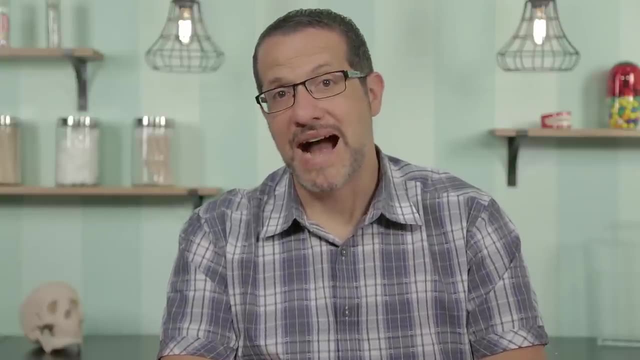 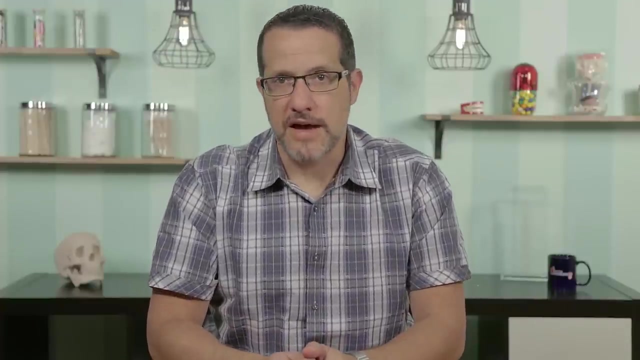 cancer mortality hazard ratio 1.17,. cancer incidence hazard ratio 1.13, and type 2 diabetes incidence with a hazard ratio of 1.91.. One study found that adults who spend six hours a day sitting and watching TV lost about 4.8 years of life. 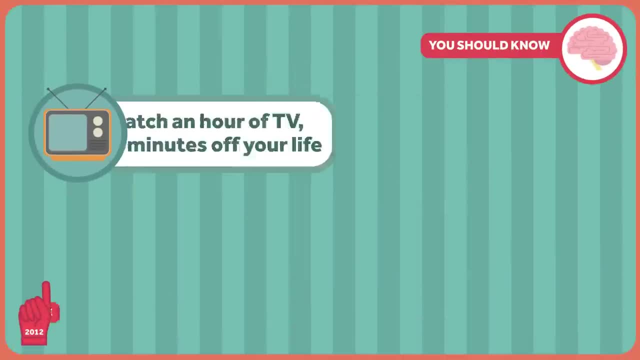 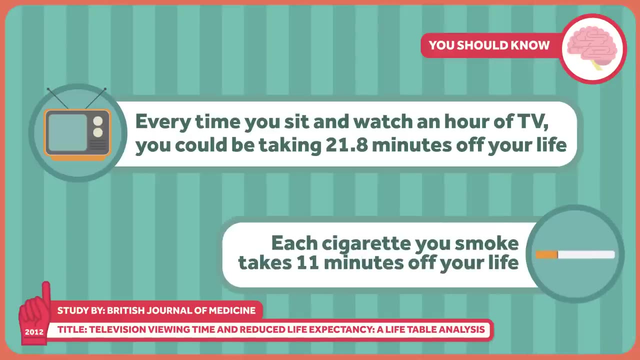 on average versus those who don't. Or you can put it this way: Every time you sit and watch an hour of TV, you could be taking 21.8 minutes off of your life. If you wanna panic, it's been calculated that each cigarette you smoke, 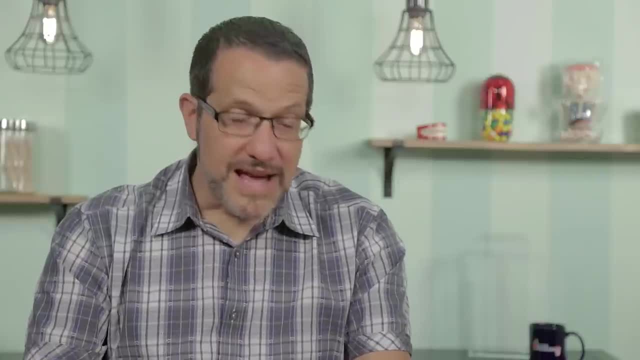 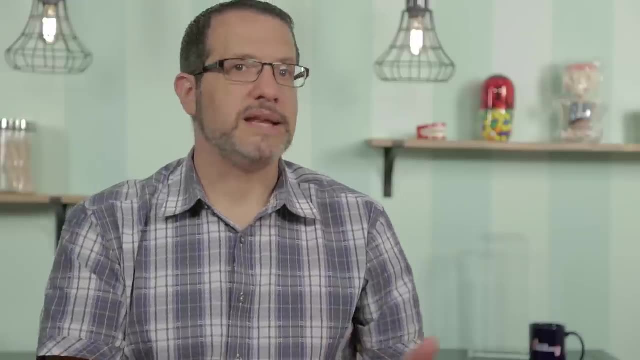 takes only 11 minutes off your life. Why is all this so? That's a harder question to answer And unfortunately we can only speculate. Obviously, some of the harm comes from sitting, leading to weight gain and obesity, which are linked to all of the diseases. 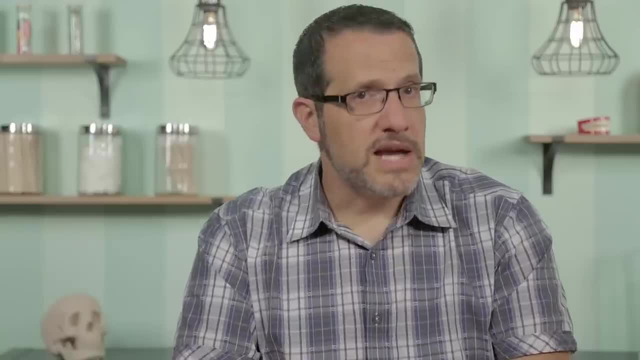 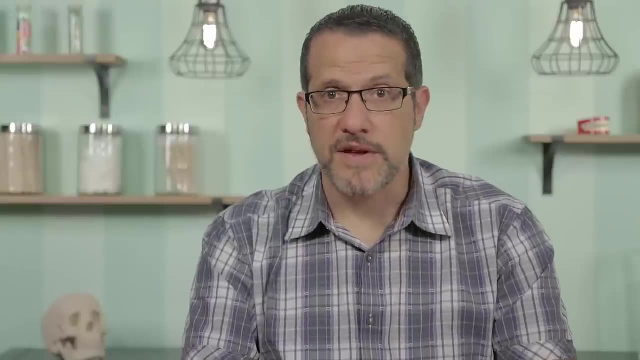 and deaths that I mentioned already, But there's likely more going on. Some scientists believe that sitting signals the body to shut off certain enzymes that help clean fats out of the bloodstream. It might also prevent the body from properly regulating inflammation and blood clotting. 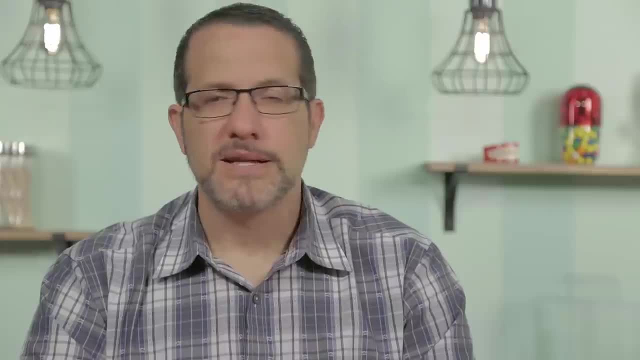 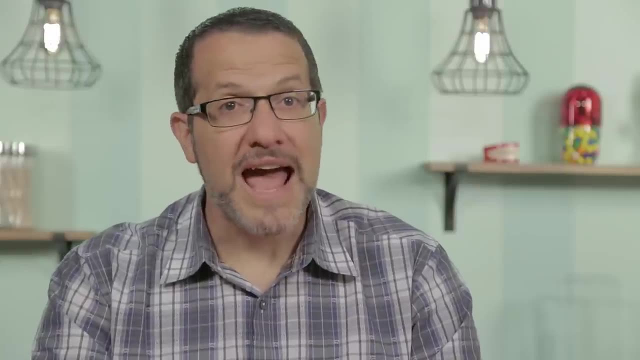 And you can't necessarily fix those things with physical activity. It's not all bad news, though. This is fixable, especially for many healthcare triage viewers who tend to be relatively young. You can not sit so much. There's research to back this up. 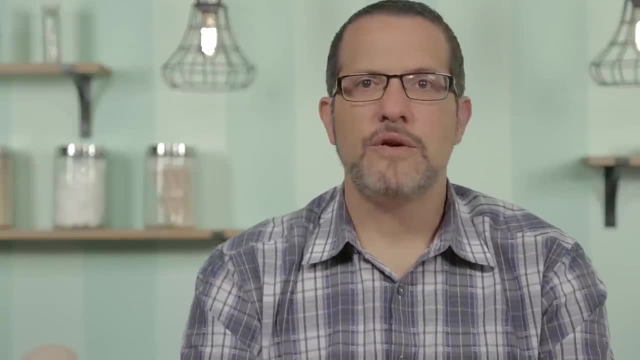 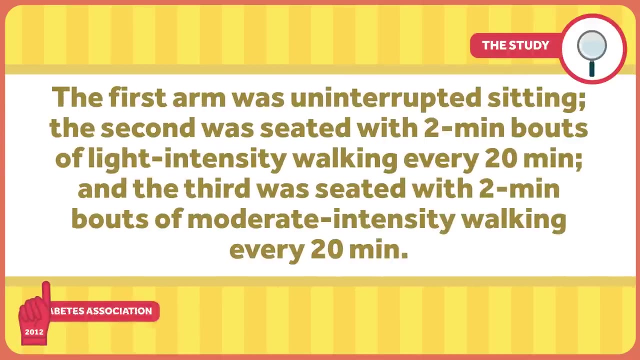 A study published in 2012 on diabetes care took 19 overweight or obese adults and put them through a randomized three-period, three-treatment acute crossover trial. The first arm was uninterrupted sitting, The second was seated, with two-minute bouts of light intensity, walking every 20 minutes. 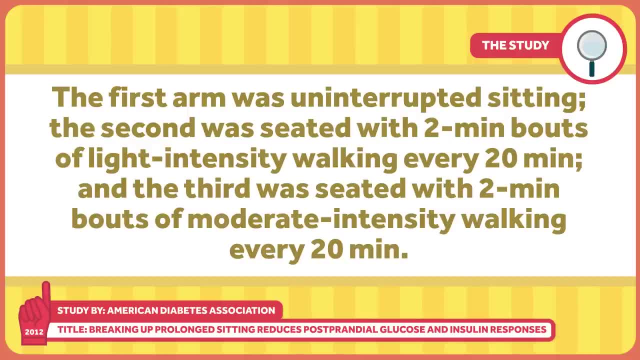 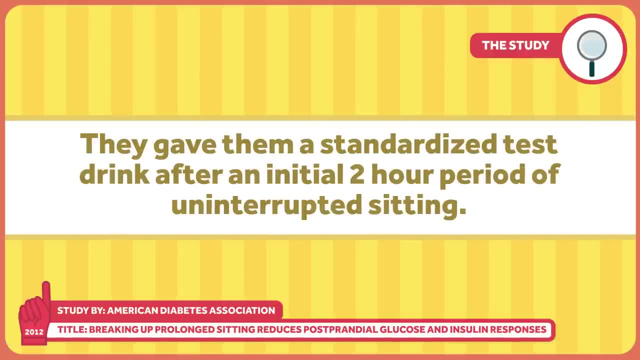 And the third was seated with two-minute bouts of moderate intensity, walking every 20 minutes. They gave them a standardized test drink after an initial two-hour period of uninterrupted sitting And then they measured their glucose levels. What did they find? That breaking up sitting time. 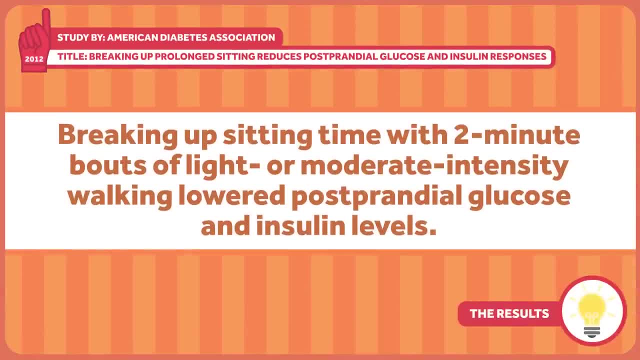 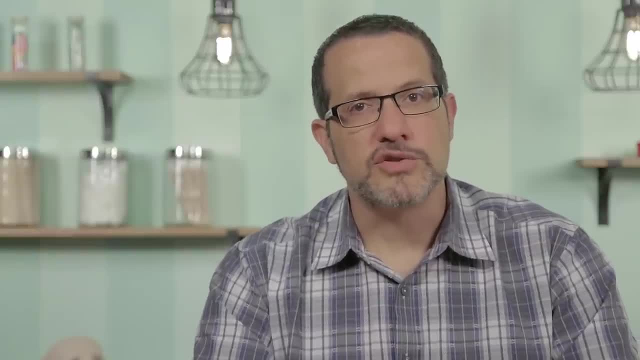 with two-minute bouts of light or moderate intensity walking lowered postprandial glucose and insulin levels. In other words, it appeared to improve glucose metabolism, which could reduce cardiovascular risk. Another study published a year later in the American Journal of Clinical Nutrition took 70 adults and ran them. 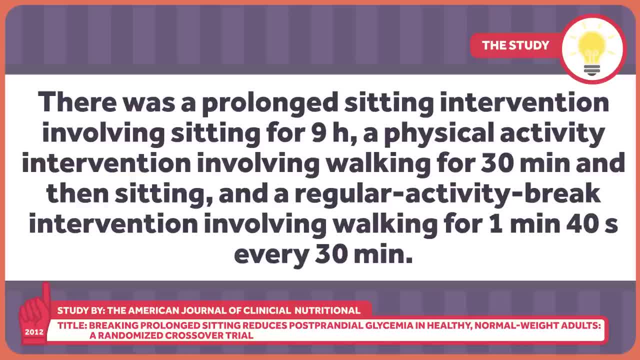 through a randomized crossover trial. There was a prolonged sitting intervention involving sitting for nine hours, a physical activity intervention involving walking for 30 minutes and then sitting for a while, and a regular activity break intervention Involving walking for just under two minutes.